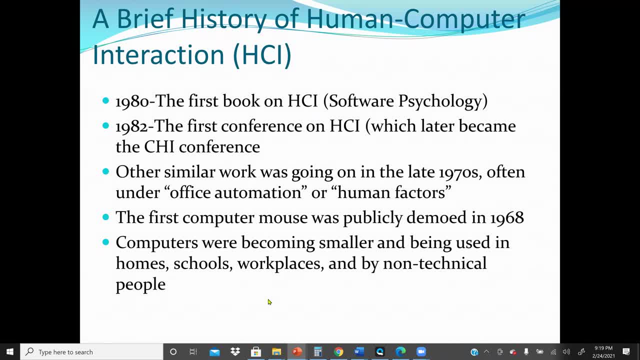 Human-Computer Interaction is developing a system that will interact with computers. A very simple example would be the mouse. So in 1968, the computer mouse was again publicly known. The computers were becoming smaller and being used in homes, schools, workplaces and by non-technical 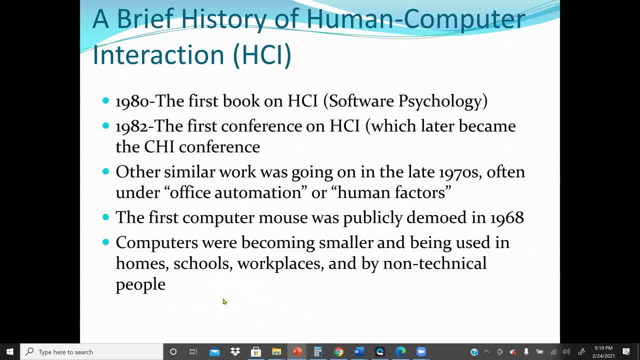 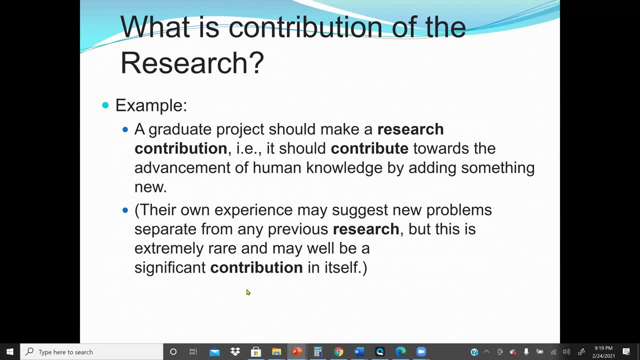 people. This was somewhere around 1980s when our first micro-computer desktop computers again started. So the first desktop computers was done by Apple Computer Company. So next, what is a contribution of the research? Again, this course is about human-computer. 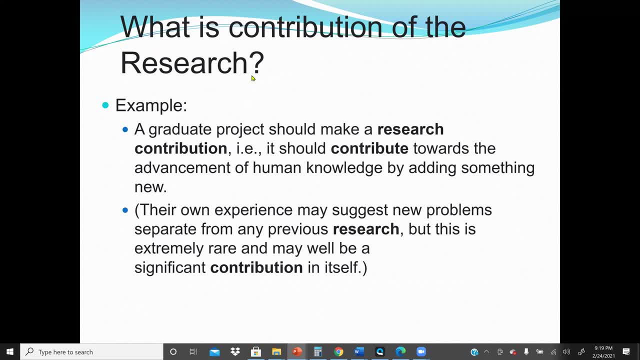 interaction research methods or, in general, computer science research method. So the first thing we want to know is: what is the contribution of a research? The contribution of the research will beif we are adding a new knowledge to a knowledge that we already know. 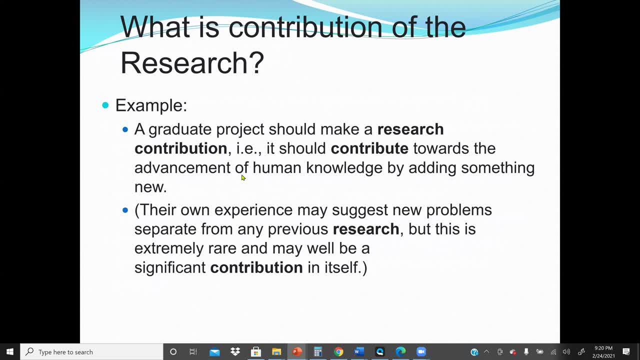 So, for example, a graduate project should make a research contribution, which means it should contribute towards the advancement of human knowledge by adding something new. So again, in human computer interaction, we have some few equipments or devices that can be used that can interact between computers and human. 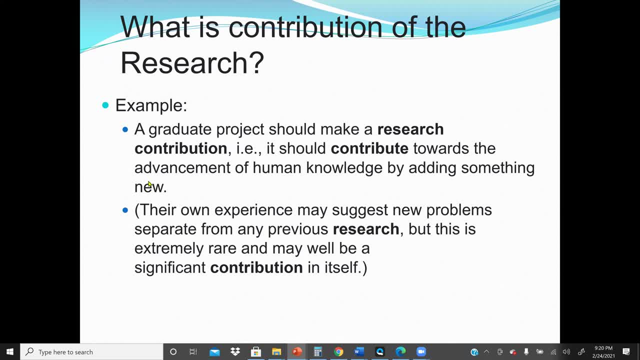 Now we may come up with a new device or develop a new system which will be more user friendly or more comfortable than previous device, And this would be a contribution to the field. So a contribution of a research means we are adding a new knowledge to already known knowledge. 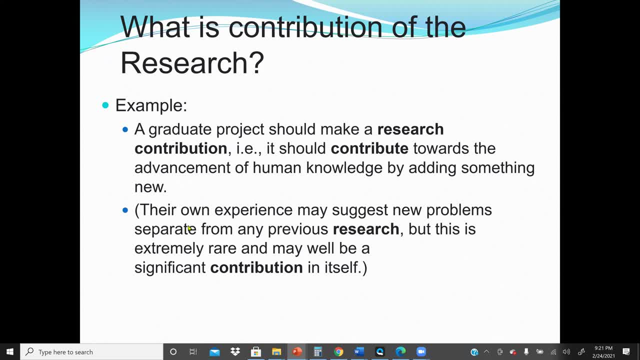 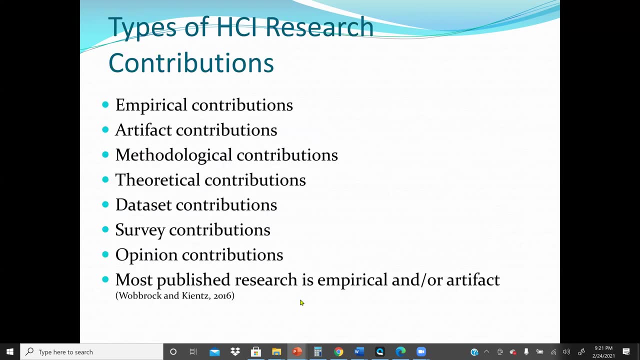 in the field, In that particular field. So their own experience may suggest new problems separate from any previous research, but this is extremely rare and may well be a significant contribution in itself. So top of HCI research contributions we have the empirical contributions. 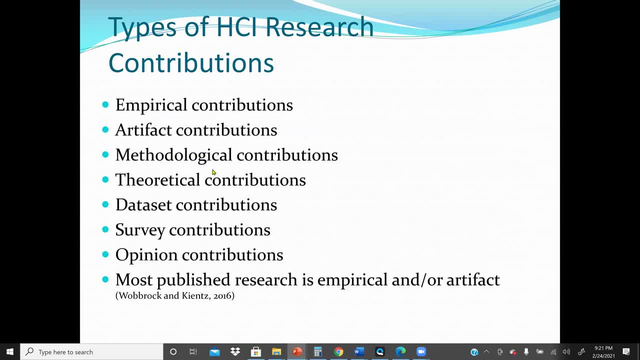 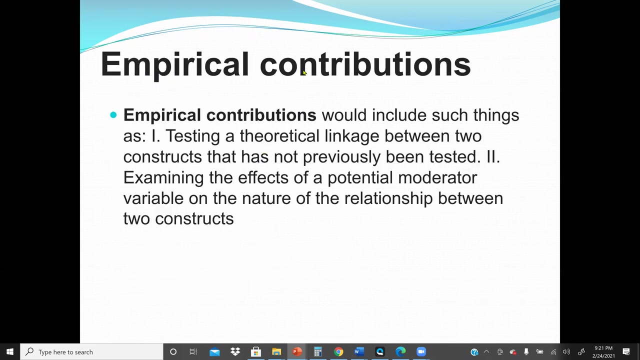 anti-fact contributions, methodological contributions, theoretical contributions, data set contributions, survey contributions, opinion contributions and also most published research in this empirical and also anti-fact, And we will go through each of these 10.. So first we start with the empirical contribution. 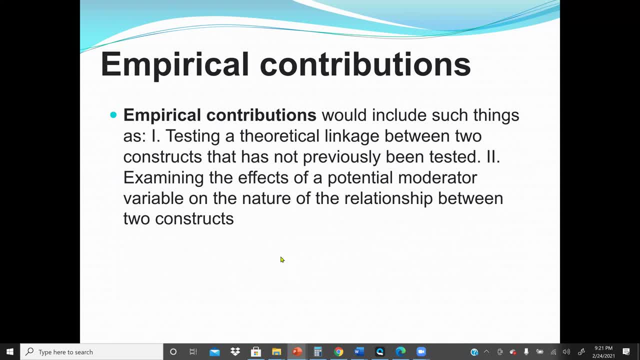 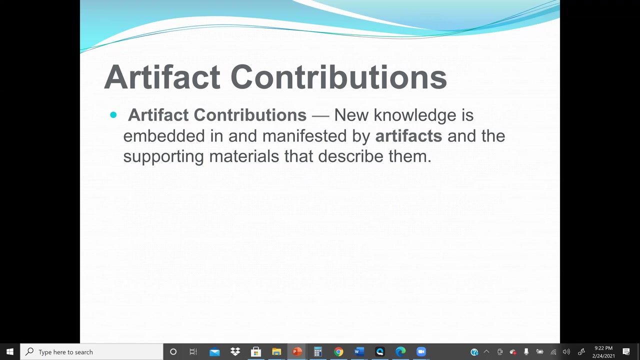 We said that empirical contribution will include such things as testing a theoretical linkage. testing a theoretical linkage between two constructs that has not previously been tested. So examine the effect of a potential moderator variable on the nature of the relationship between two constructs. Then anti-fact contribution is a new knowledge is embedded. 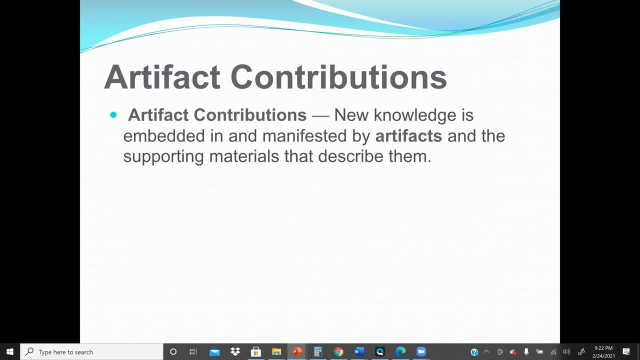 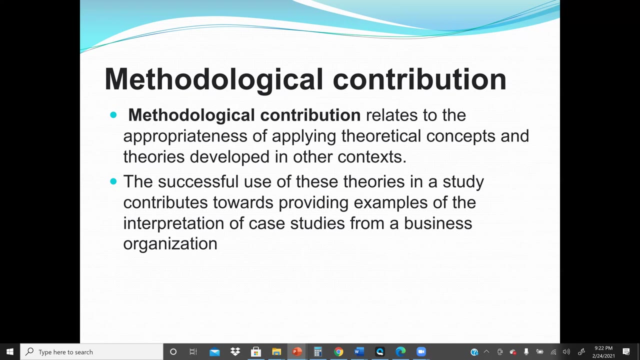 in or manifested by anti-facts, and the supporting materials that describe Then will be again anti-fact contributions. Then we also have methodological contributions, which will be related to the appropriateness of our prime theoretical concepts and theories developed in other contexts. 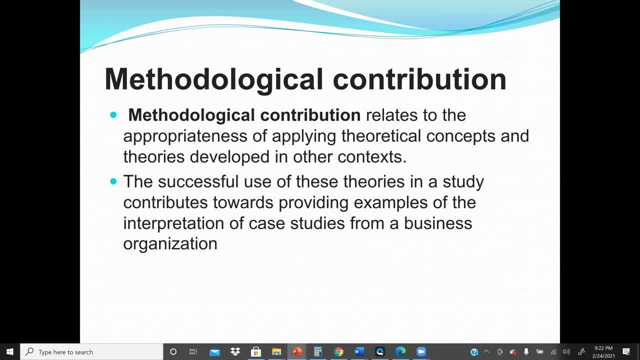 So the successful use of these theories in a study contributes toward providing examples of interpretation of case study from a business organization. So again, methodological contribution will always relate to the appropriateness of applying some method or theoretical concepts and also theory developed in other contexts. 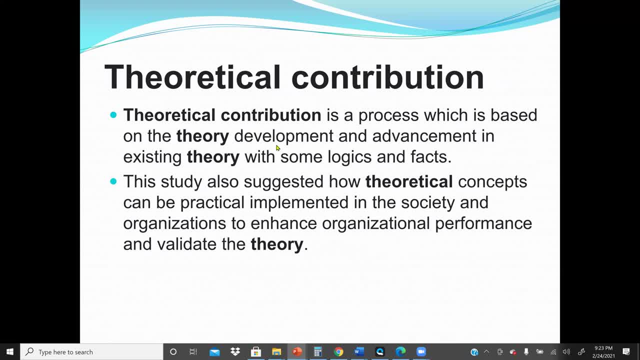 Theoretical contribution is a process which again is based on the theory development and also advancement in existing theory. We saw logic, We saw theory development, We saw logic and facts. So this study also suggested how theoretical concepts can be practically implemented in a society and also organizations. 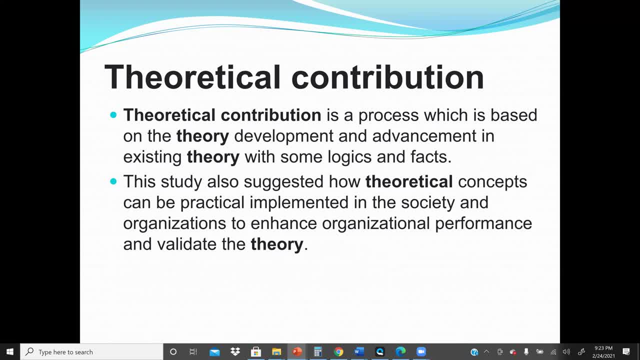 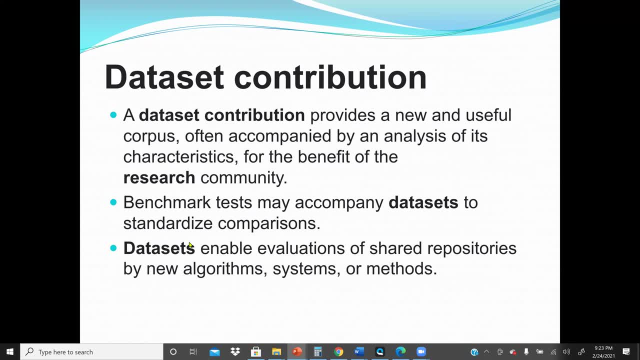 to enhance organizational performance and validate the theory. We also have the data set contribution, which provide a new and also a useful corpus, often accompanied by analysis of history. We also have the data set contribution, which provide a new and also a useful corpus, often accompanied 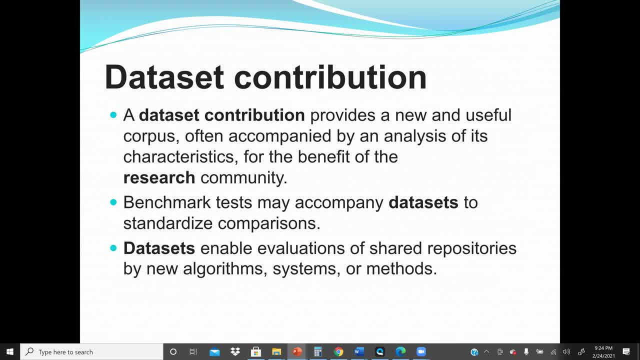 by analysis of history. So in case of a student who is in a Inte-Houkai or a university that has trouble in a science program that is a major or a major research program, that we provide a new data set. that is an easy way to download a data set. 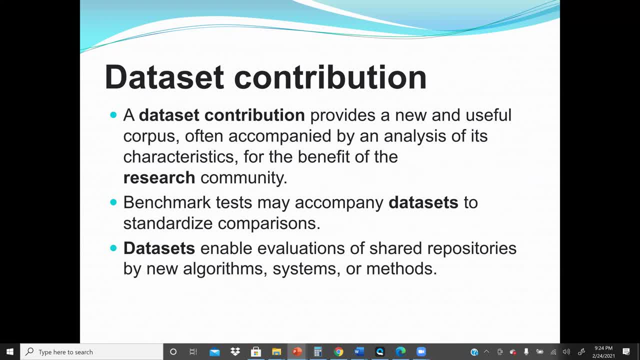 The data set is also a tool for the evaluation of findings in the research community. So an example will be a benchmark test may accompany a data set to standardize comparisons. So a data set again enabling evaluation of a shared risk-based theory by new algorithms, systems or, again, methods. 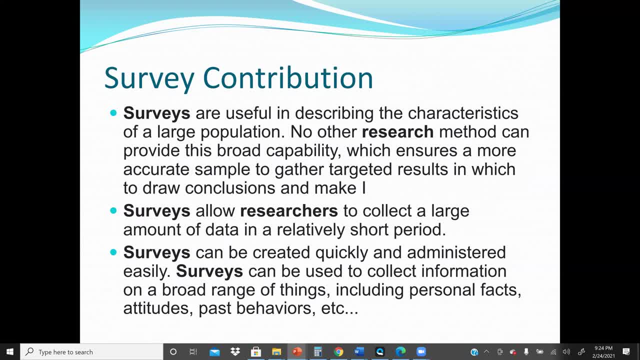 A survey contribution again are very useful in describing the results And the data set is a way to also generate results. So when we use a data set, again this is very useful in describing contribution again are very useful in describing the characteristics of a large population. 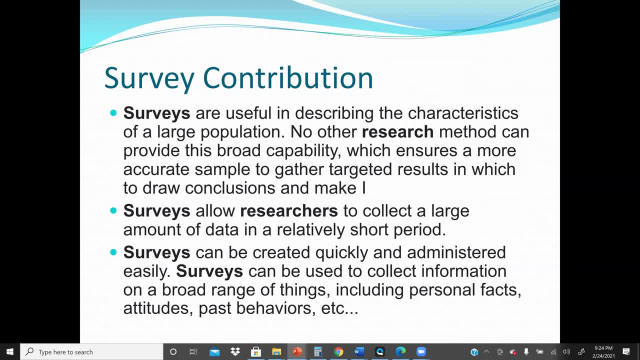 so no other research method can provide this broad capability. and most of the time again, when we are conducting the research, we use sample instead of a large population. so this again shows a more accurate sample together targeted result in which to draw conclusion, and this conclusion again will be applied to the population, to characterize the population. so 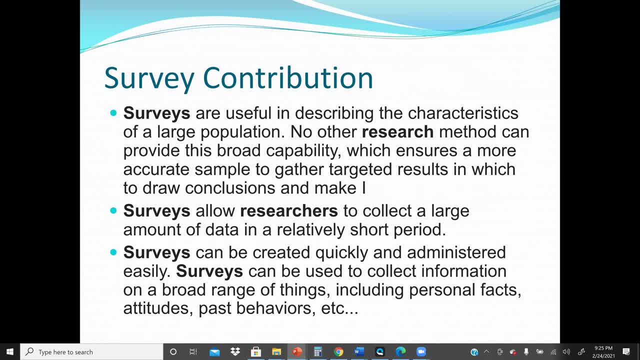 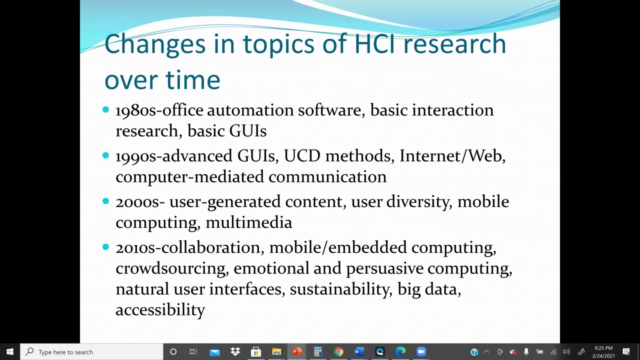 surveys allow researchers to collect a large amount of data in a very short period of time and also surveys can be created quickly and also administered easily. surveys can be used to collect information on a broad range of things, including personal facts, attitudes, past behavior etc. so changes in topics of acr research over time. somewhere in 1980s we have office automation. 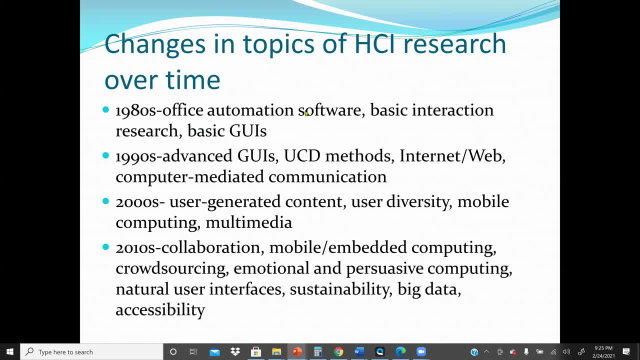 software, which is the basic interaction research or basic graphical user interfaces, going then by 1990s. we have advanced goings. graphical user interfaces also use ucd methods, internet, web, computer mediated communication. we have touch screen censuses. we can use sensors to again interact with computers. this is normally using games. 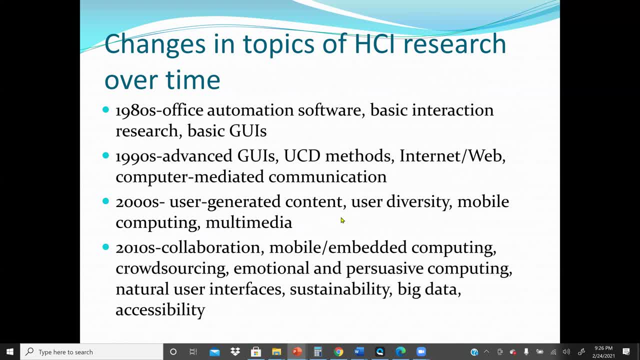 by 2000 the user generated content, user diversity, mobile computing and multimedia became common. then by 2010s, we have a collaboration system where we may have two people or two locations, different sites all together. they can they get through a software system, collaborate and adapt, work together or play together. we also have a mobile embedded computing. 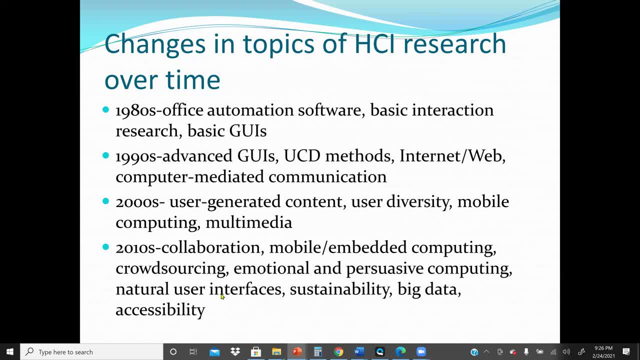 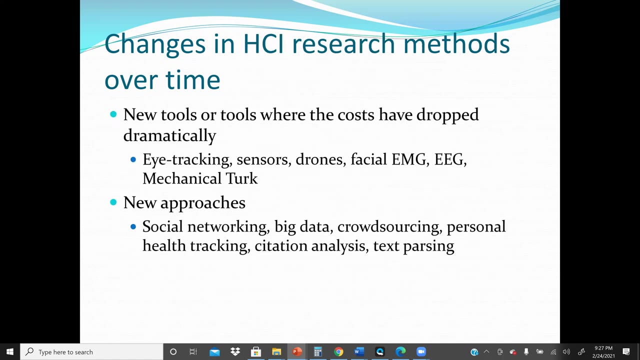 system. we also have the crowdsourcing: emotional and persuasive computing- this regard to robotic interaction with robot systems. also, we have the natural user interfaces: sustainable sustainability, big data and accessibility. so changes in hci research methods. over time it's a new tools or tools where the costs have dropped dramatically. 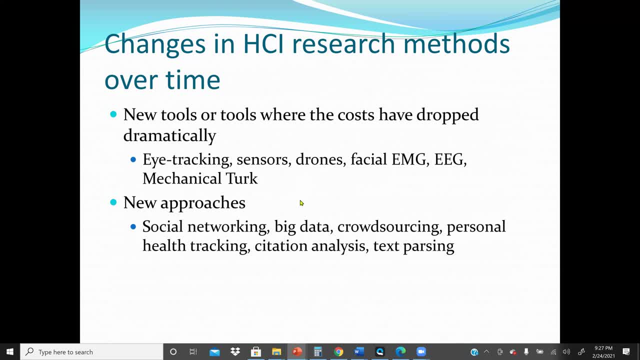 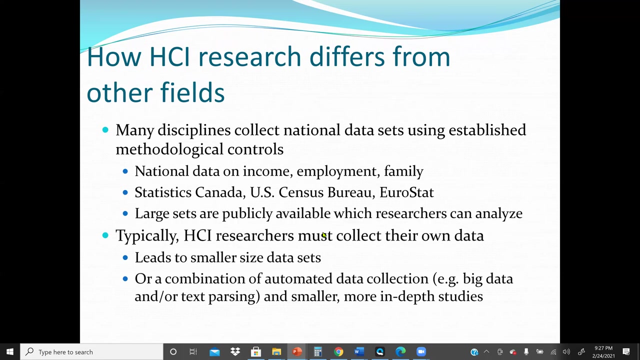 example can be the high tracking sensors, drones, facial, emg, eeg, mechanical talks. and new approaches now will be social networking using big data analysis concept, crowdsourcing, personal health tracking, citation analysis and test passing. so how hci reset differ from other fields? yeah, we know again many disciplines. 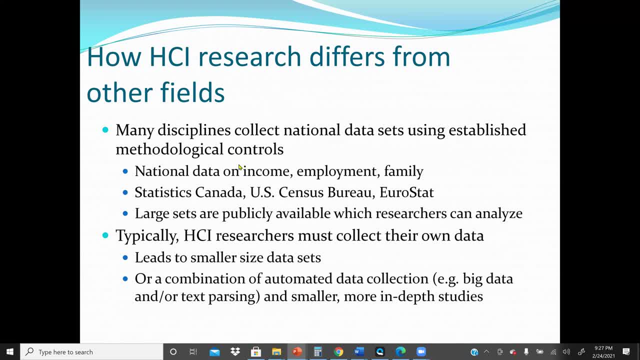 collect national data set using established methodological controls. example will be national data on income or employment family. we also have a statistics canada or us census bureau, eurostat. again, most of these disciplines use a data collected- national data set- to establish a concept or methodology. so life sets. 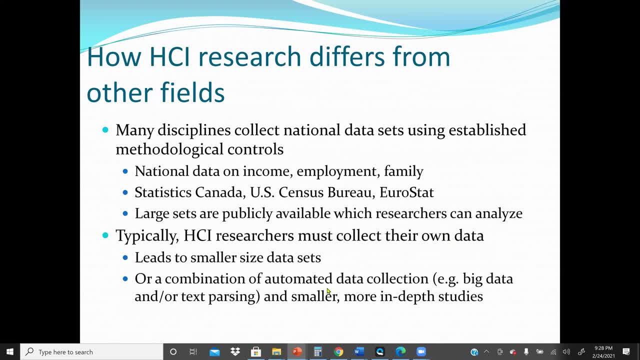 are publicly available which researchers can analyze. typically, hci researchers must collect their own data instead of using an existing data. this will lead to a smaller size data set or a combination of automated data collections. example would be a big data and or test parts and smaller, more detailed studies. 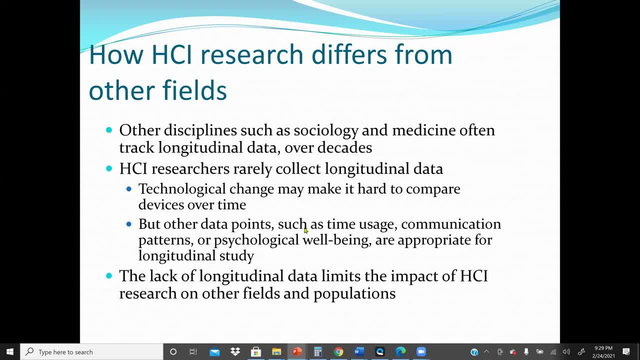 other disciplines, such as social networking, will allow the goal of mass research to be more inclusive or to identify the basic needs of the research facilities with the team. other disciplines such as social networking will also allow the goal of mass research and sociology. medicine often track data that's based on period of time. 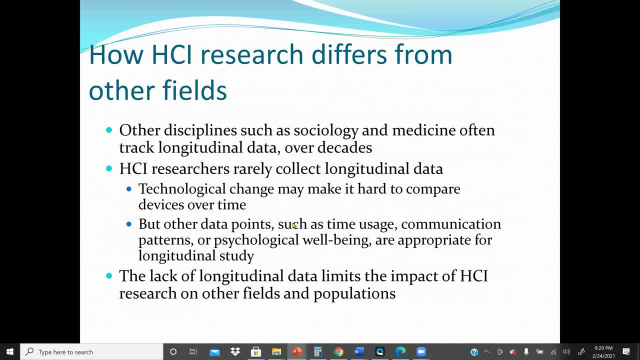 longer than that data- over decades- Then HCI researchers rarely collect data that's for a period of time. Technological change may make it hard to again compare devices over time. Again, HCI is another emerging field and very dynamic field. So collecting longitudinal data- that's, the data within some long period of time- 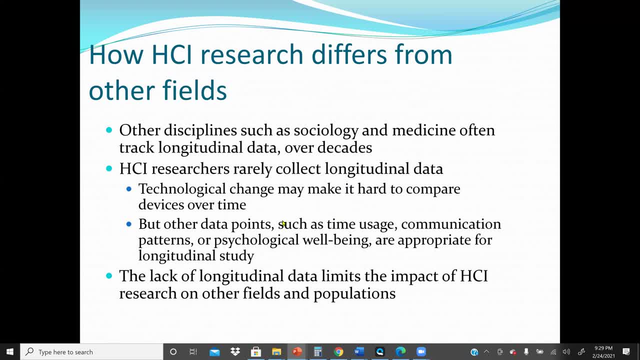 would not be a benefit for HCI, But other data points such as time usage, communication patterns or psychological well-being are appropriate for longitudinal studies. Then the lack of longitudinal data limit the impact of HCI research on other fields and also populations. Now how HCI research differ from other fields. 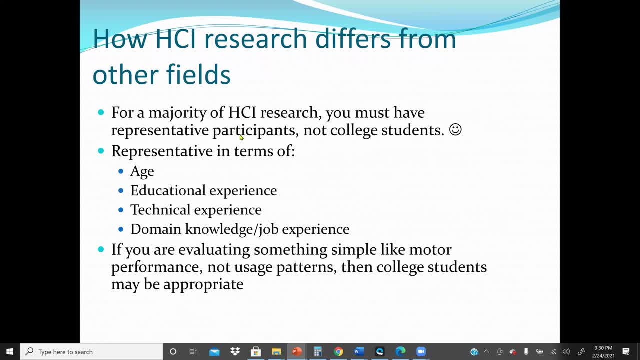 Again, majority of HCI research. we must have representative participants, not college students, So representative in terms of HCI research. we must have age group criteria of age or educational experience, technical experience, domain knowledge and job experience. The main reason again that we know HCI is more technically involved. 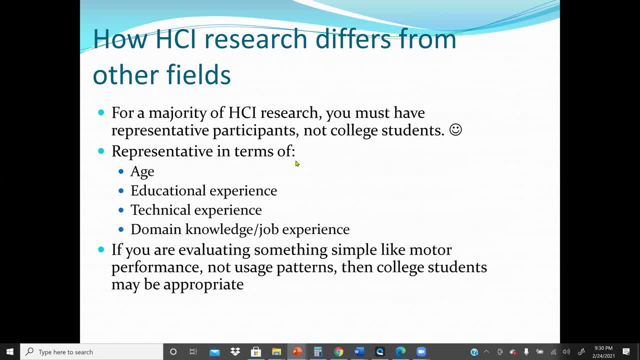 having the participants that have a knowledge about the technology, and also by age. Maybe we may try to develop a system that will interact with case to print again. So this will be based on age. A complex system maybe will be based on technical experience. 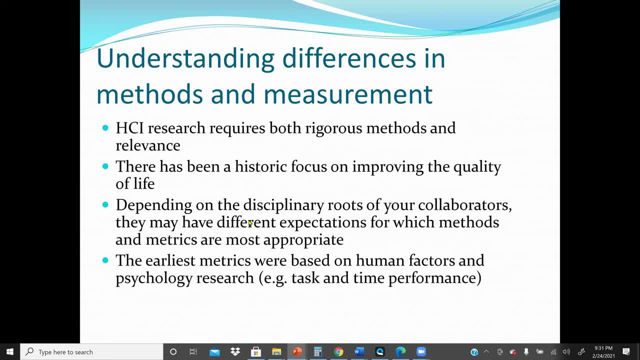 of the participants, et cetera. So we should understand the difference in methods and measurements. HCI research require both rigorous methods and relevance. Also, there has been historical figures on improving the quality of life. Now, depending on the disciplinary roots of our collaborators, 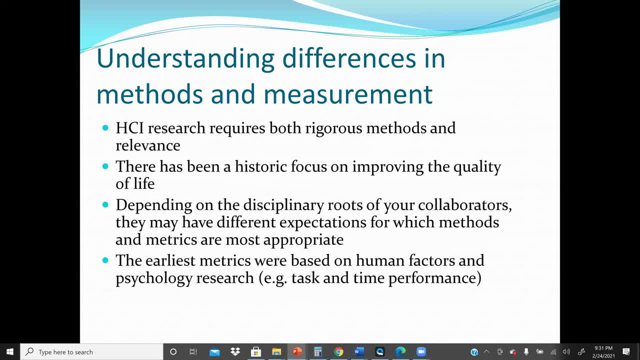 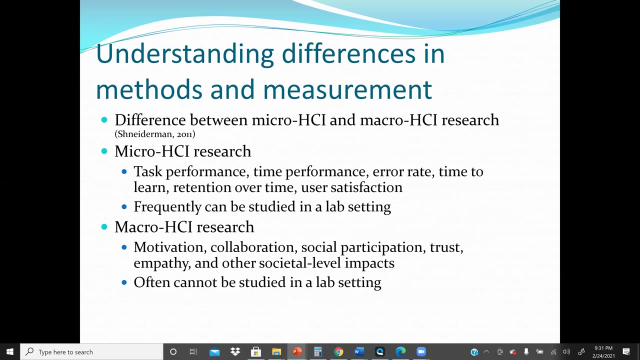 they may have different expectations for which methods and metrics are most appropriate, And the earliest metrics were based on, again, human factors and psychological research. A good example would be tax and time performance. Now, the difference between micro HCI and macro HCI research is that 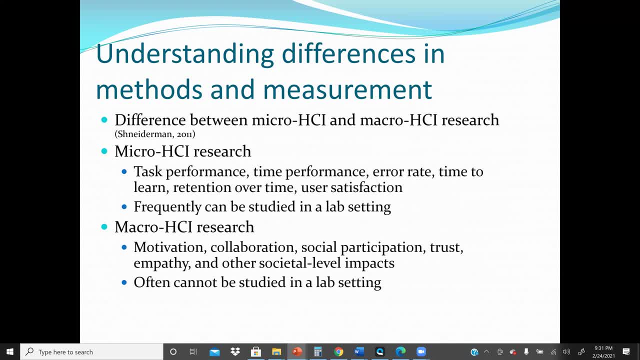 a micro will be something that varies significantly. So a micro HCI research will be a tax performance, time performance, error rate, time to learn, retention over time, user satisfaction and frequently can be studied in a lab setting. But micro HCI research will be based on motivation collaboration. 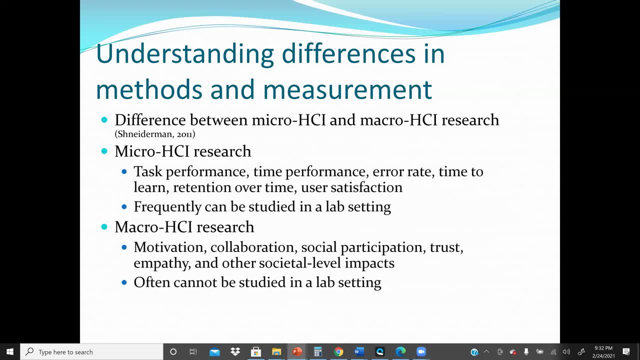 because, again, this is a large research, So a collaboration, social participants, trust, empathy and other societal level impacts. This often cannot be studied in a lab setting because it's a large research platform. So the nature of interdisciplinary research in HCI. 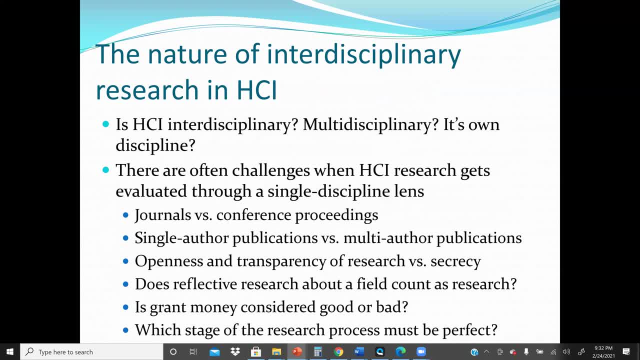 is HCI interdisciplinary or multidisciplinary, or its own discipline? So yeah, we said that there are often challenges Where HCI research gets evaluated through a single discipline lens, For example, journals versus conference proceedings. We have a single author publication versus multi-author publication. 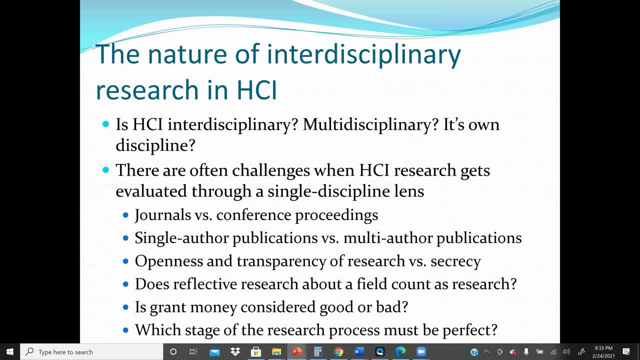 Openness and transparency of research versus secrecy. Does reflective research about the field count as a research? Also, is grant money considered a good or bad? Which stage of a research process must be perfect? Now, who is the audience for our research? 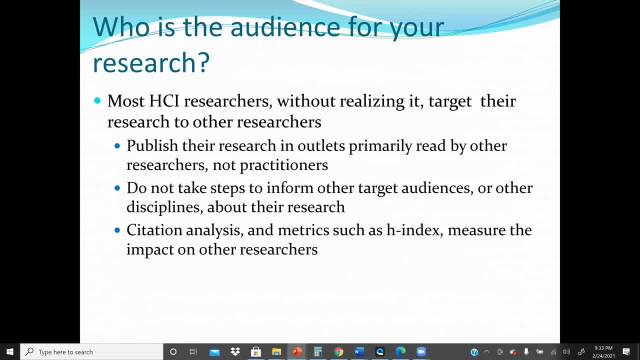 So most HCI researchers, without realizing it, target their own research to other researchers. They publish their research in outlets primarily read by other researchers, not practitioners. Also do not take steps to inform other target audiences or other disciplines about their research. Citation analysis and metrics such as H-index measure the impact on other researchers. 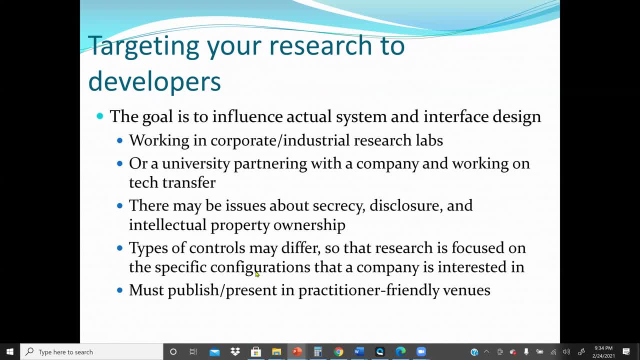 Now targeting your research to developers is. a goal is to influence actual system and interface design. So working in a corporate or industrial research labs or university partner with a company and working on tech transfer. Also, there may be issues about secrecy, disclosure and intellectual property ownership. 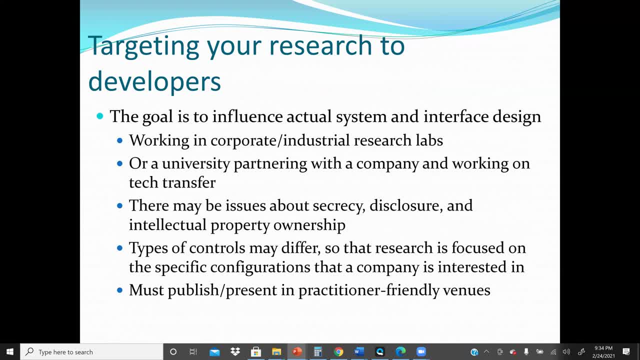 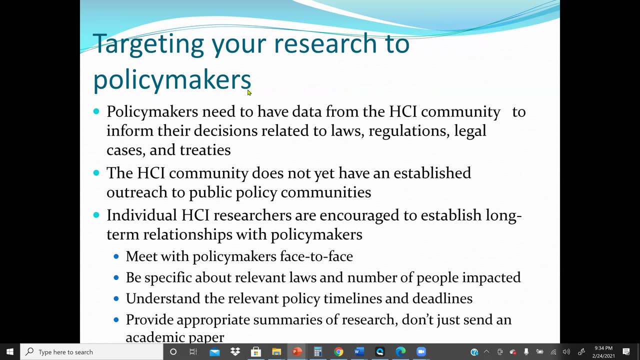 Also, types of controls may differ so that research is focused on a specific configuration that a company is interested in Must publish and also present in practitioner-friendly values. Also targeting research to policymakers. So policymakers also need to have a data from HCI community. 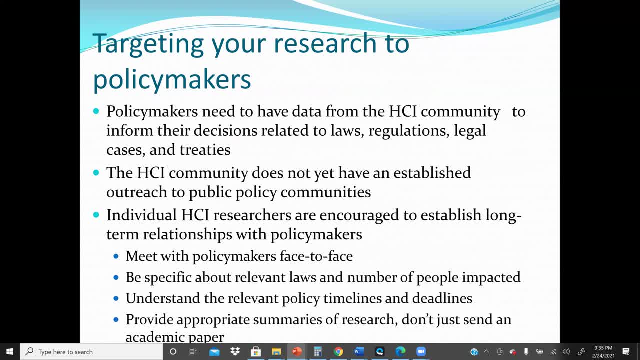 to inform their decision related to laws, regulations, legal cases and treaties. So HCI again committee does not yet have an established outreach to public policy communities. Individual HCI researchers are encouraged to establish long-term relationship with policymakers. Meet with policymakers face-to-face. 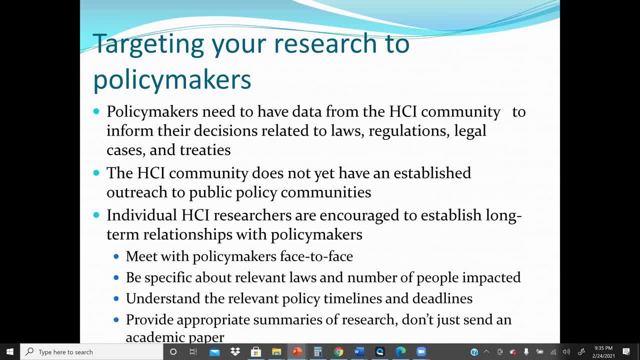 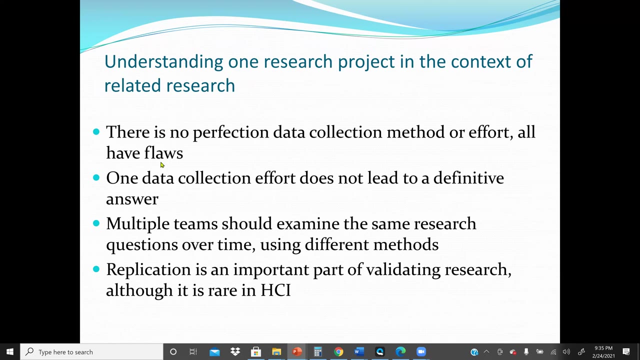 Be specific about relevant laws and number of people impacted. Also understand the relevant policy timeliness and deadlines. Provide appropriate summary of research. We should not just send an academic paper Understanding one research project in the context of research. so we know there is no perfection, data collection method or effort. 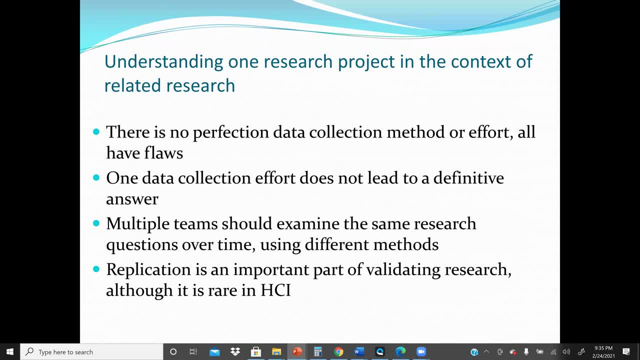 Or have a fraud. One data collection effort does not lead to a definitive answer. Multiple teams should examine same research questions over time, using different methods. Replication is very important, So it's an important part of validating our research, Although it is rare in HCI. 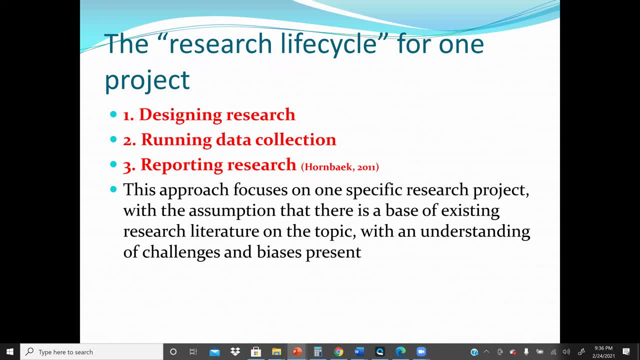 So research life cycle for one project: We can start with the designing the research, Then running the data collection, Then reporting the research. So this approach: focus on one specific research project, With assumption that there's a base of existing research literature on the topic. 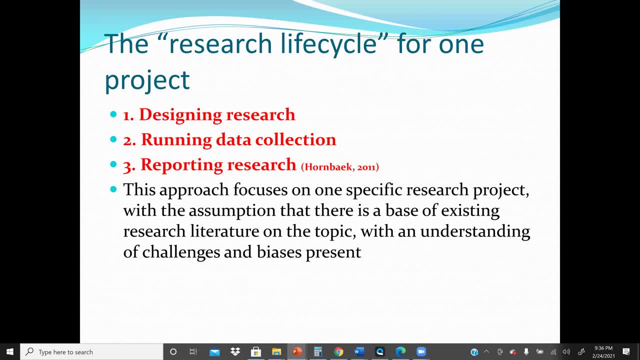 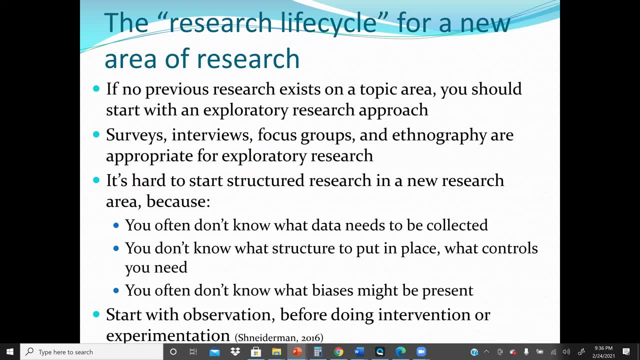 With an understanding of challenges And biases present. So a research life cycle for a new area of research. If there's no previous research exists on the topic area, Then we should start with exploratory research approach. Again, in this case there's not a background literature review. 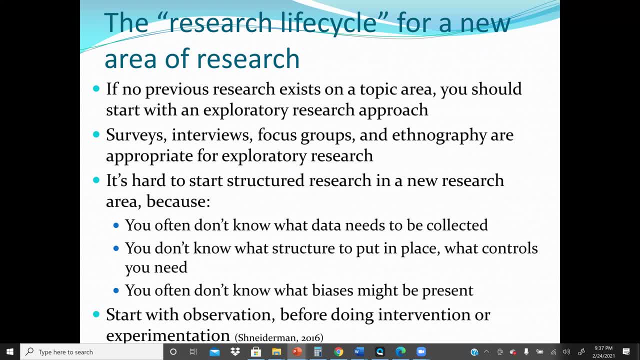 It's a new research. So exploratory data or exploratory research Approach makes us to understand Our research question And also the new, the phenomena we are studying. So surveys, interviews, focus group Ethnographic are appropriate for exploratory research. 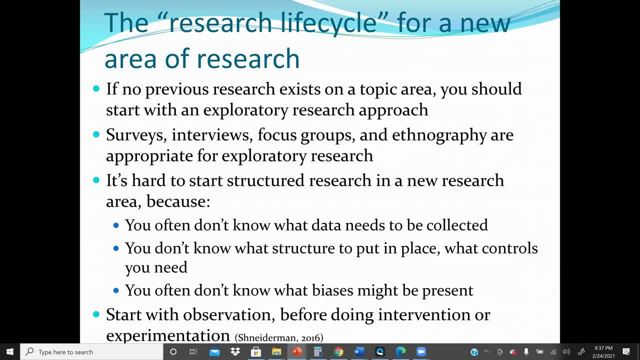 And also it's very hard to start structural research in a new research area Because You often don't know what data needs to be collected. You don't know what structure to put In place, What controls we need. You often don't know what biases might be present. 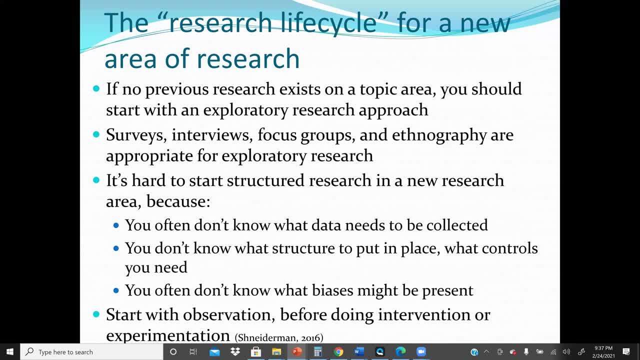 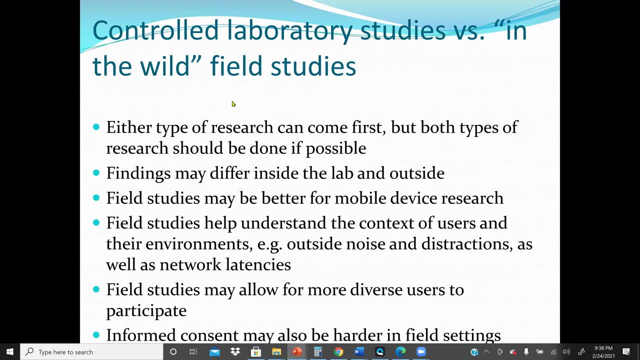 So we should always start with exploratory Approach and also with observation Before doing intervention or experiment. Also, the control lab, laboratory studies vessels in a wide field studies. So either type of research can come first, Either laboratory studies or, But both types of research should be done if possible.